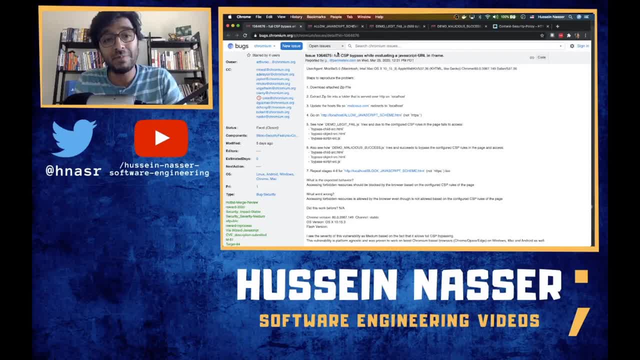 So it looks like there is a bug in Chrome that allows certain individual to bypass content security policy, which is pretty dangerous. We can talk about it, guys, because the bug has been fixed and has been closed and has been installed in the latest version of Chrome, So we can publicly talk. 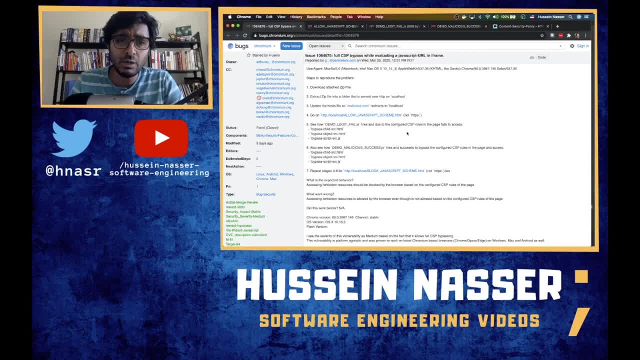 about it. The fix is there, So no longer zeroed in. How about we talk about it, guys? We're going to discuss what content security policy is. what was this bug exactly and how did this? whomever discover this? And I think they're going to get a reward as a result: Golf clap for finding great. 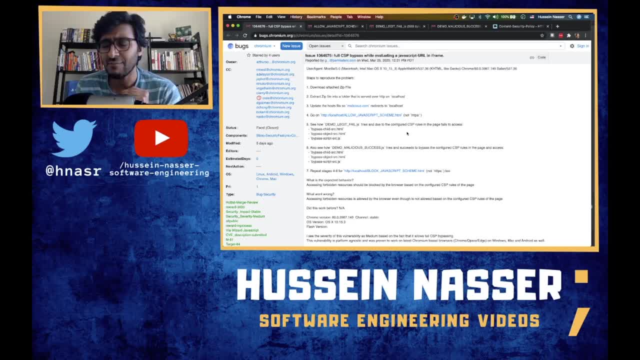 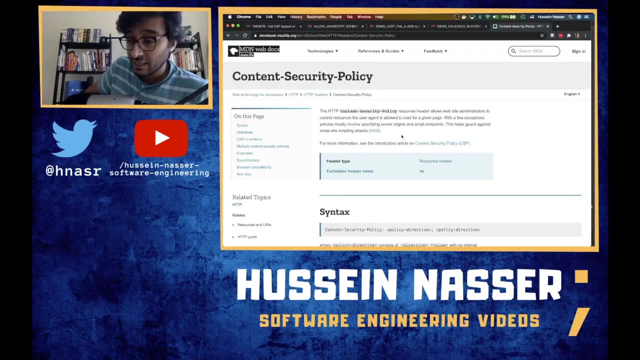 bug? I don't think personally. it's a major, big, high severity bug, but I'm going to leave that decision up to you guys. So how about we jump into it, guys? What is content security policy? We talked about that, guys, in the 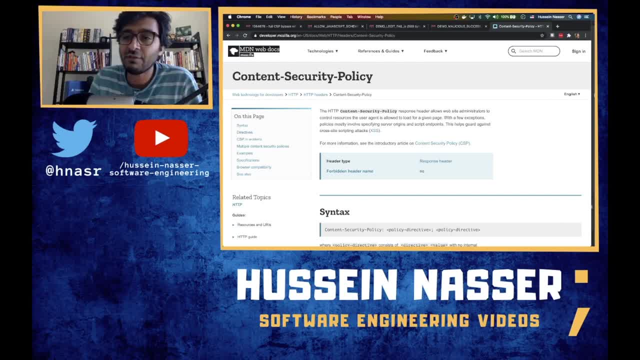 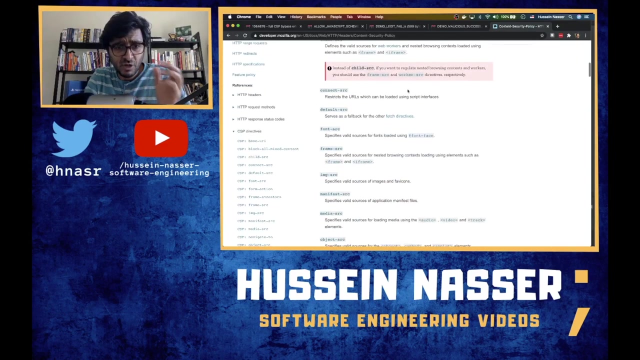 cross-site scripting video. Check out the video right here. But essentially what it is is in a given page. you can set certain policies to load images, to load object frames, scripts, to only load them from certain sources. right, And we talked about that. For example, there is a default. 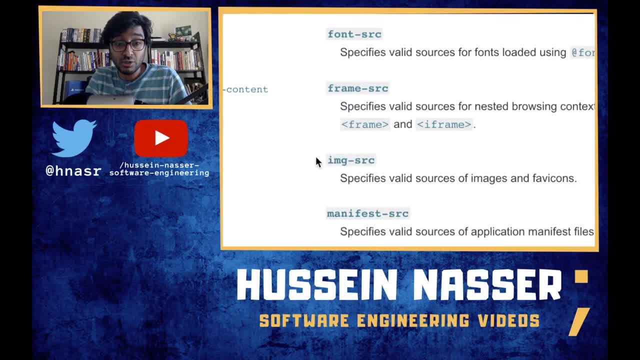 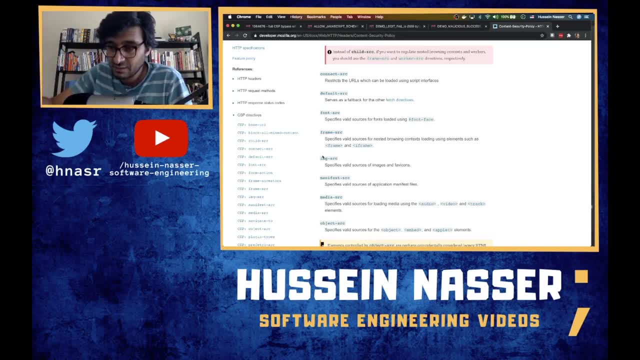 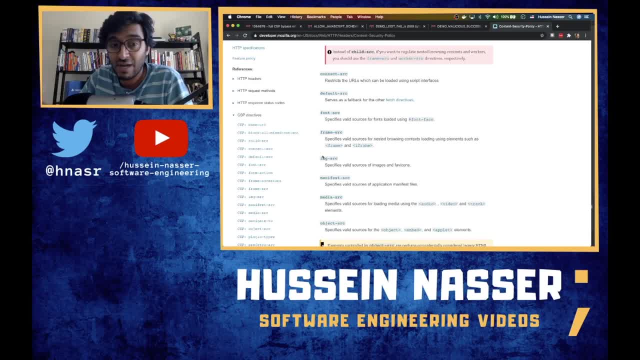 domain right. If there are images coming from other domains, please do not send, get request to that URL because it's most likely it's an XSS attack. right, The cross-site scripting, And we talked about how dangerous this is: A single image tag that. 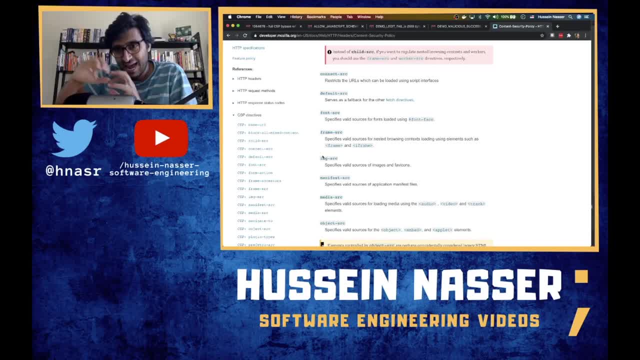 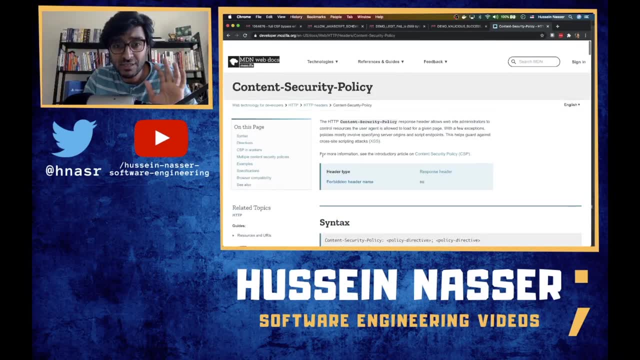 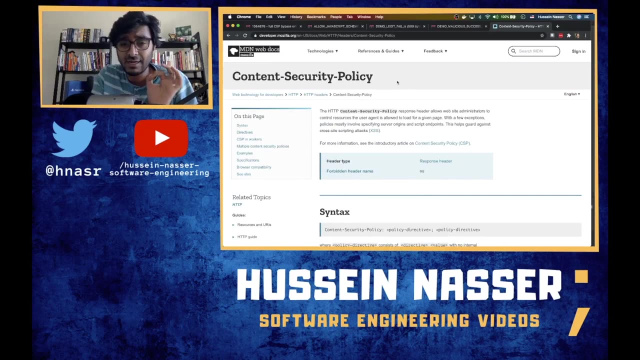 It's really an image. It's a get request to a slash that actually just sends your cookies right to that destination. So it's bad. So content security policy, it's pretty, pretty, pretty good stuff. We can set it either in the metadata, a meta tag right of the page itself, Like: let me. 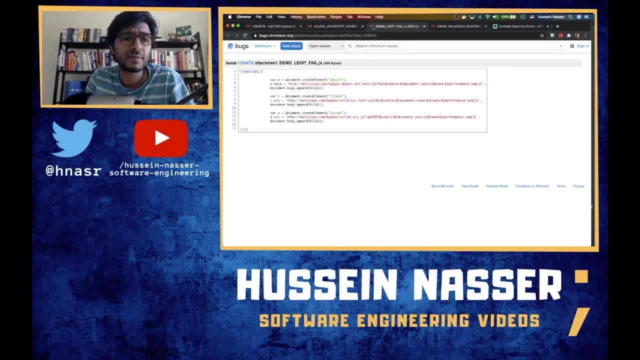 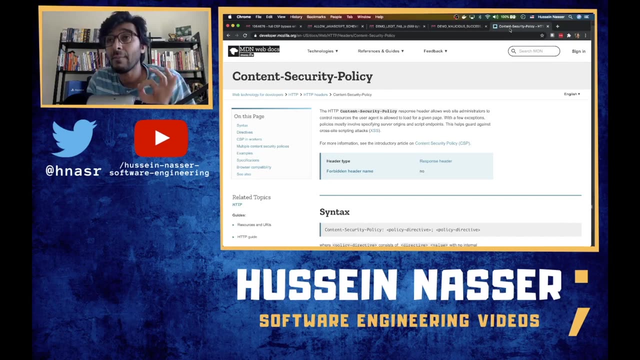 show you an example- Not here, Not here. Like here, You can set it as part of a meta tag Or, as backend engineers, we can set it as part of the payload headers coming back from the server. So as you start building the page or building the content, it doesn't have to be an HTML page. 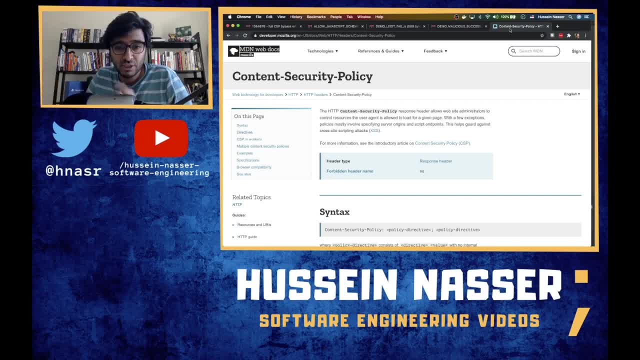 right, You want to set these headers So the content, security policy headers, So that, hey, scripts from this document should only come from this, for example, Or not in line. Don't do a just random script. that's the worst thing you can do. right for XSS, it's like this is the. 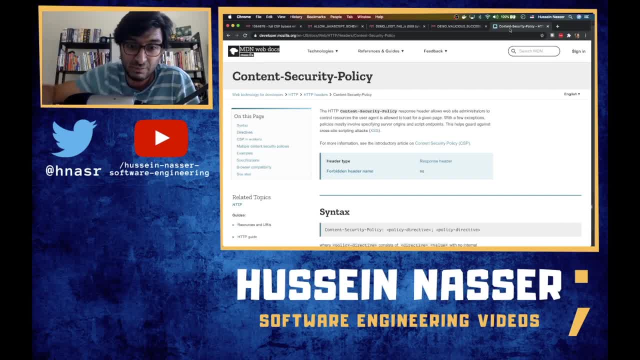 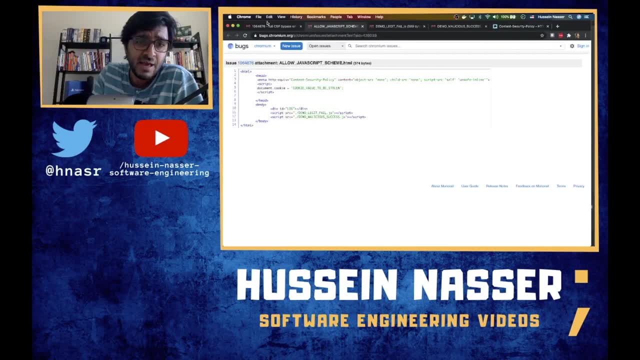 easiest thing to make it for people who want to inject scripts in your page, just right, so avoid that stuff altogether. Now let's come to the bug that has been found. the bug is actually a bypass. no matter what content policy you do, this person found a way to bypass this. 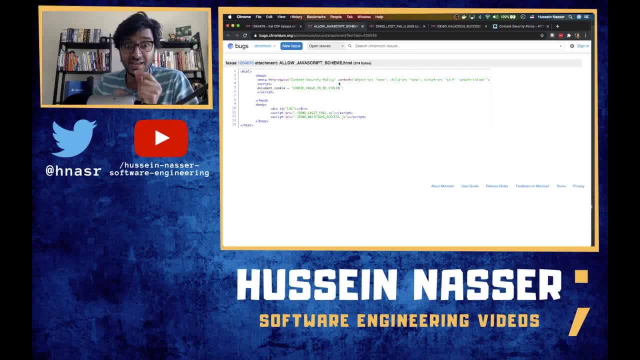 as content security policy, so that he was able to execute code that he shouldn't have be- or she doesn't have to be, right, yeah, so let's get into it. so I'm gonna warn you that it's not really easy to execute this attack because, first of all, 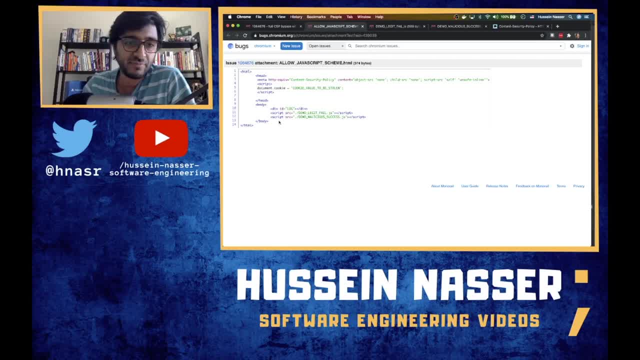 let's go through the attack first, and then I'm gonna explain why it's not that serious in my opinion. so here's the page that they have given HTML. he said: no source child, no script and no frames, so nothing should be executed. right and no inline. 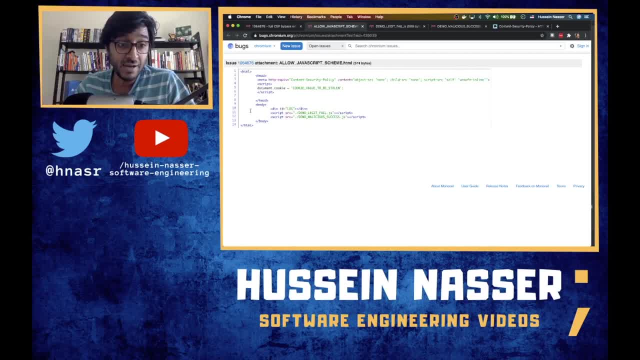 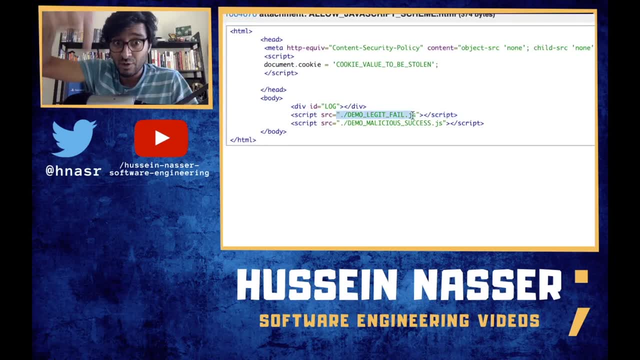 right, anything should come from the same script. and he's here in the HTML. he's loading two scripts, right? the first script, which is loaded from the same domain, and that's okay. right, because we're loading it from the same domain and he's loading it from the same domain. 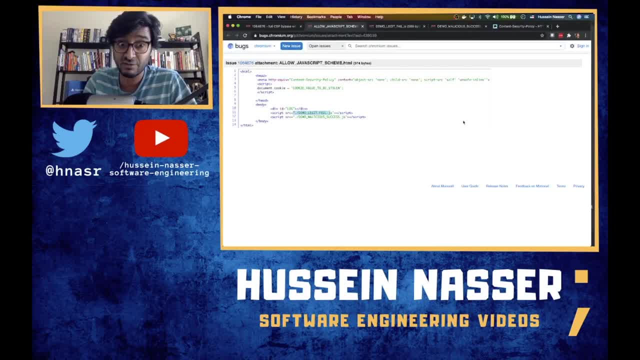 right, and that's okay. right because we're loading it from the same domain, and that's okay. we said self is okay, script executing from the self domain is okay. so this script will be loaded. this script will be loaded. but let's look at the two scripts that. let's look at the 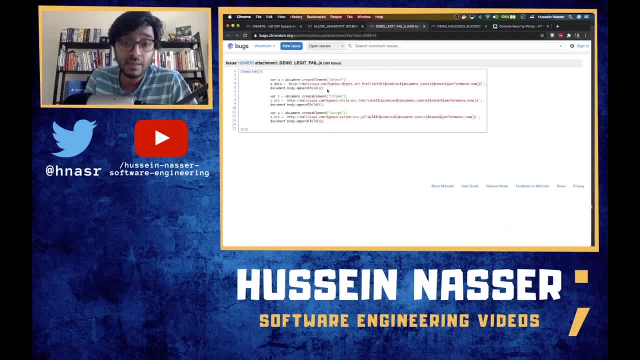 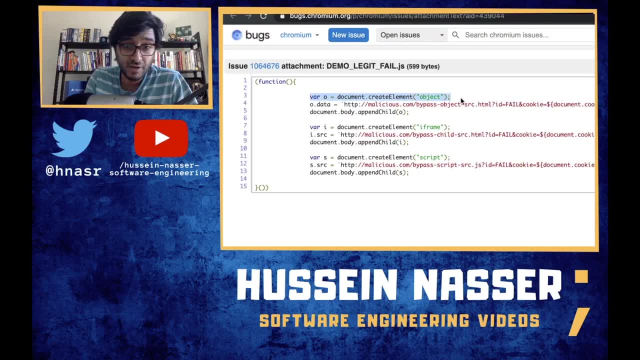 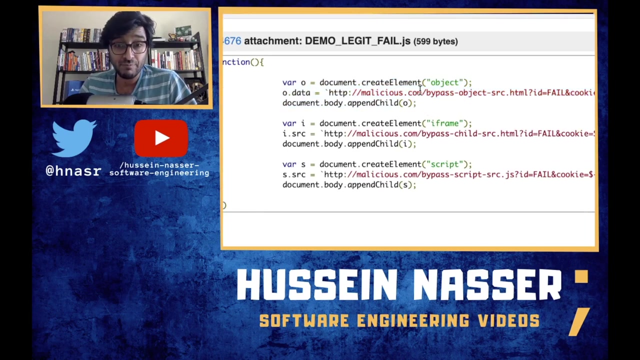 legit fail script. the legit fail script does this. it immediately executes a function. right. with this code, you create an object, which is not no problem. you can execute any script you you want, because those scripts right are, are are belonging on the same page, technically right. but this shouldn't be a uh uh should not be applicable. why? because you're creating an object. 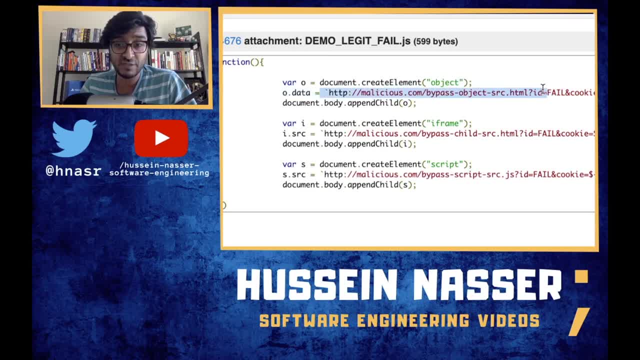 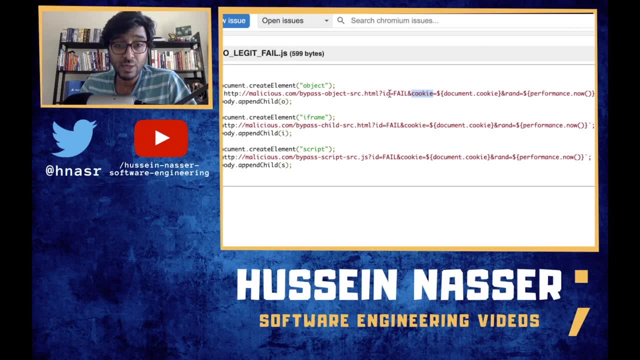 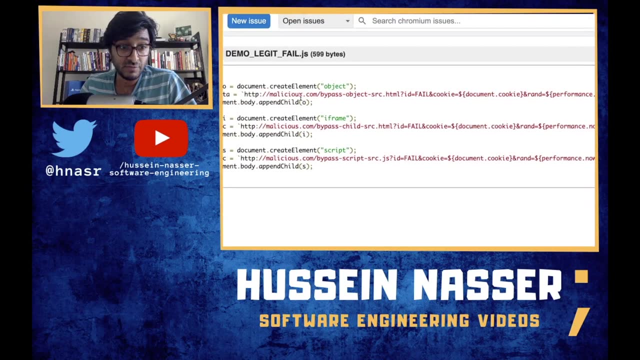 and you're inserting the data to be a completely different url. so he's he's using a get command essentially to do a, a, a, a u r l parameters and send the cookie document, which is the javascript code, and he's using, of course, text, obviously the text stuff, right? so so he can just inject that stuff and he's just. 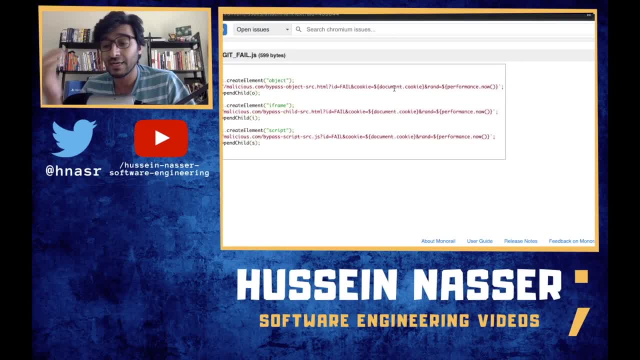 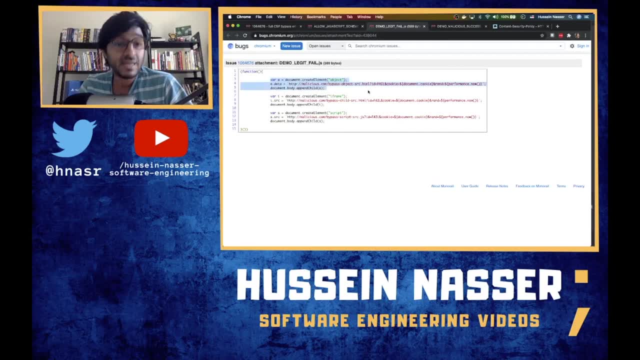 sending the cookie, assuming that this is only going to be, uh, not http, only cookies, right? only the javascript stuffy. so yeah, he's using that. so this is failing. this is failing. this is: this is failing. this is failing. this is failing. there is a point here that this is not疫. 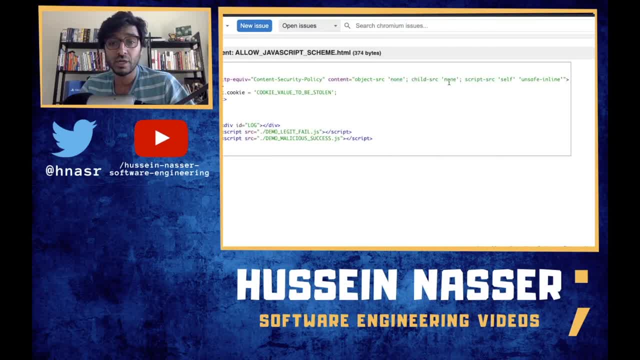 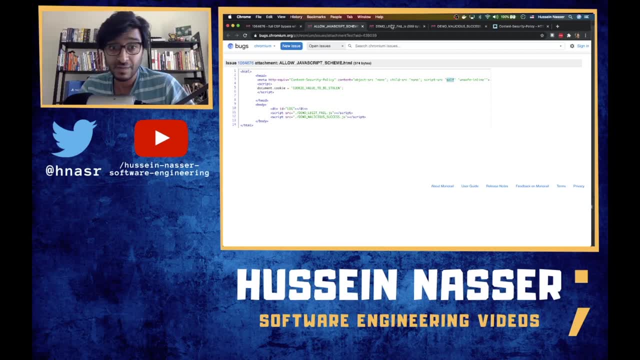 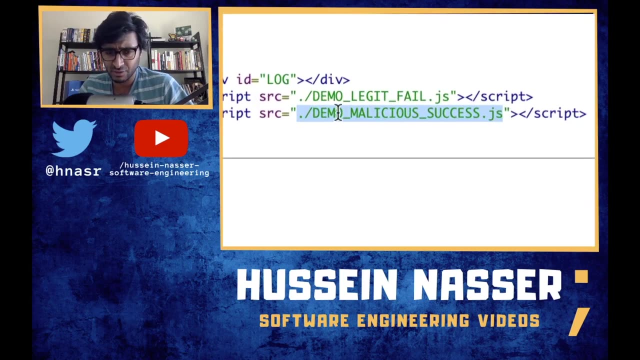 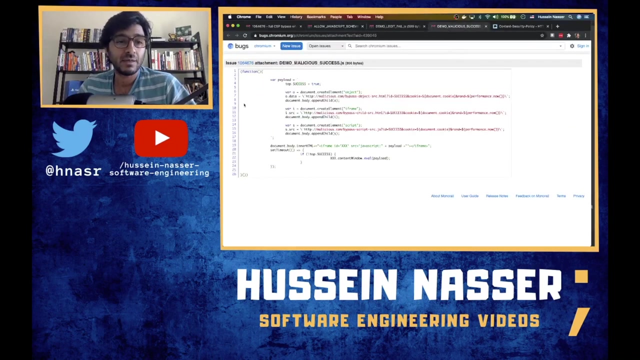 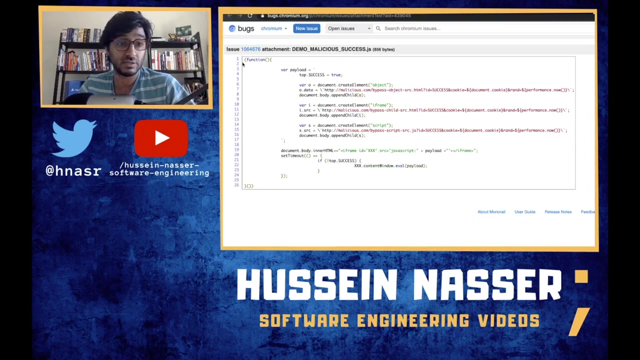 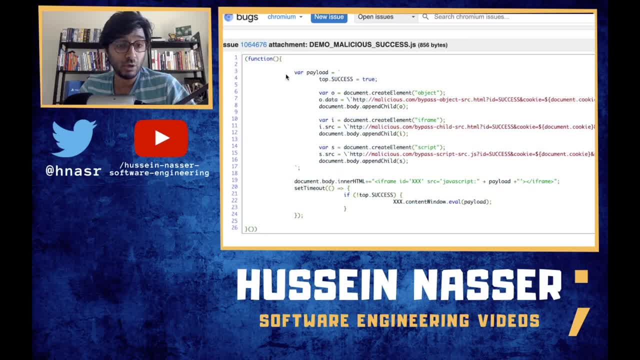 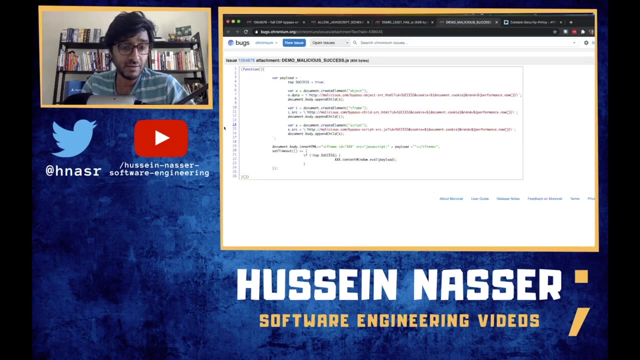 so again, that function, no problemito, you can do this. but look what he did. he created just a beautiful big payload of string, which is the same code that he basically wrote. here i keep saying, hey, he, okay, they right, so they did that and they put all of that string as a payload. so to to the 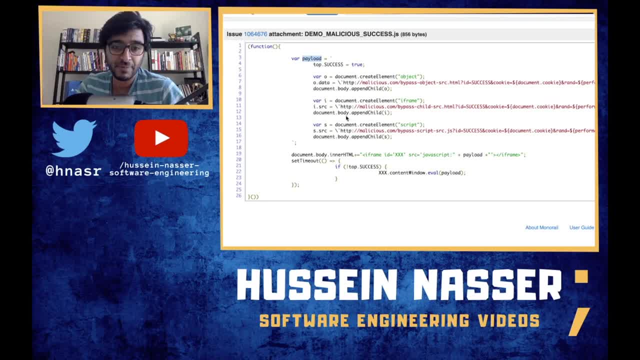 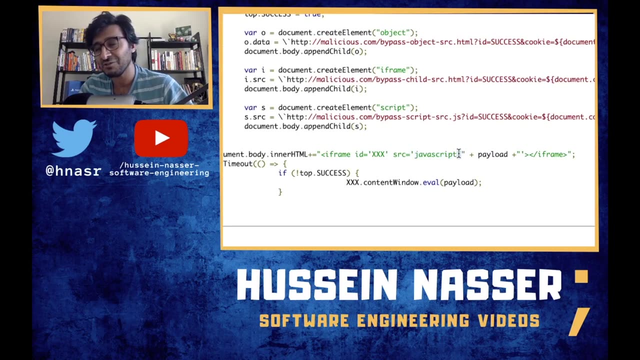 javascript executing. it's just a bunch of a string, right. and now he, uh, they, they put the inner html, and then he, they use the iframe, and then did the javascript calling which i use so many times back in the 90s- my god, i use this so much- like. 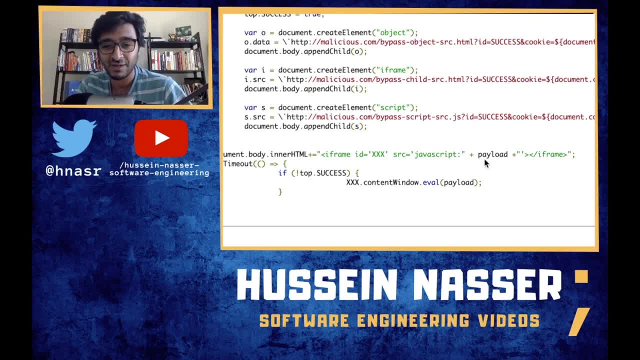 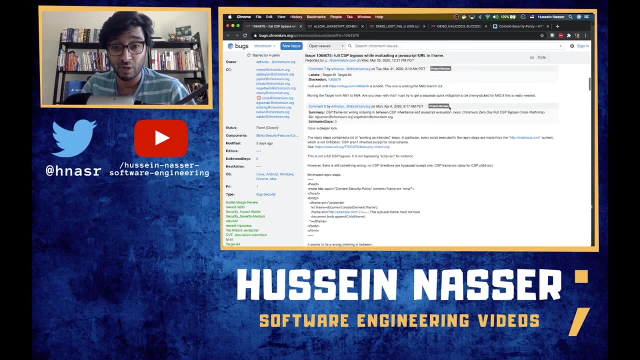 javascript colon on click. i always used to do this right. this basically execute, opens a browser brand new document. That's what it does, And I got this not from my ass, obviously, I was reading this. The smart people commented here, the project members. essentially, Let's give some props to. 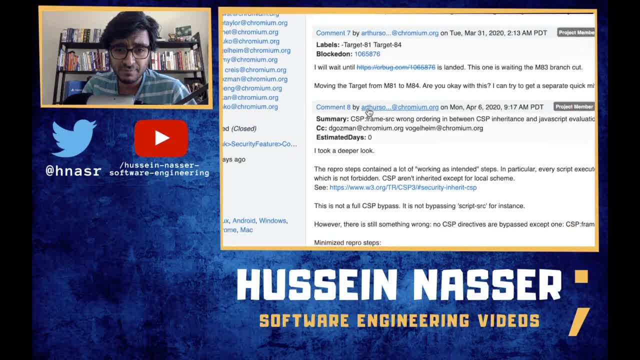 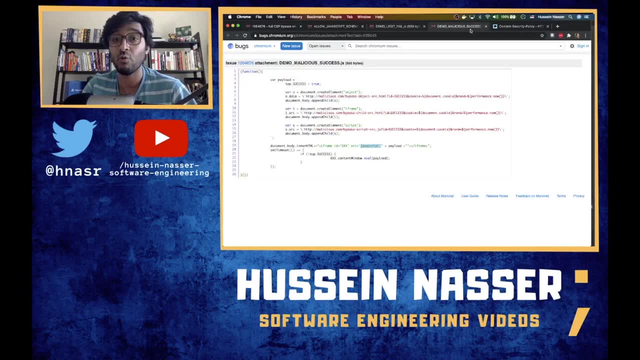 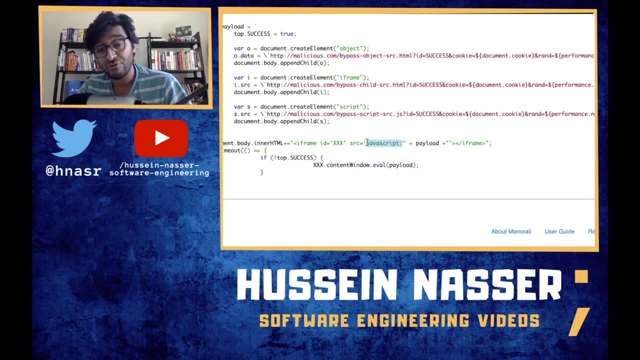 people. What was his name? His name is Arthur. I think so Arthur, but his name is not. I think his name is Arthur. So, yeah, he's the guy who found the fix and fixed it, obviously. Yeah. So what the JavaScript parameter does? it takes the payload, which is a string. 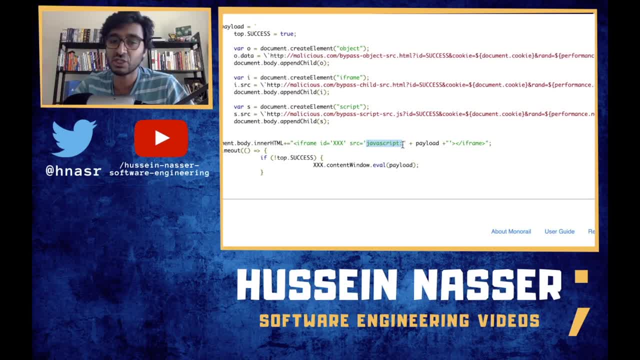 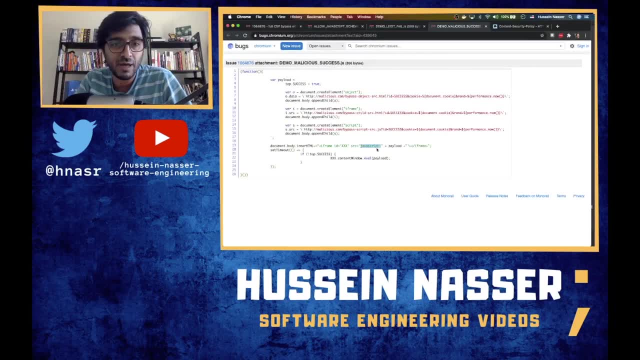 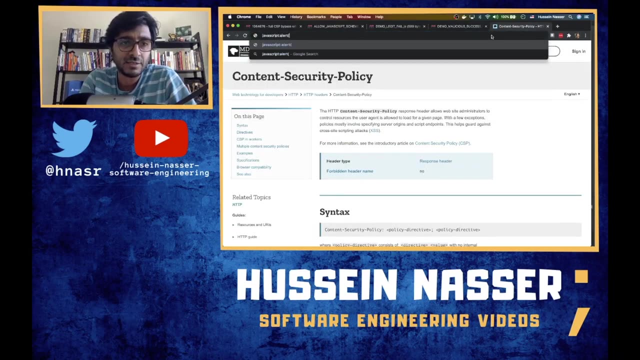 and it executes the code, Whatever it is. it just executes it. But when it executes it, it opens a brand new blank page, just like we do with the browsers. like this: right, If I do, let's do it right here. If I do, JavaScript alert test right And I hit enter. 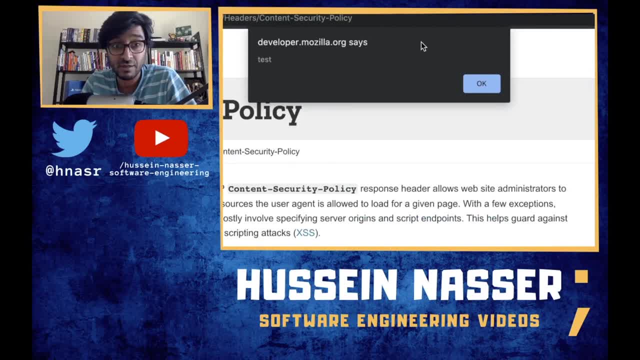 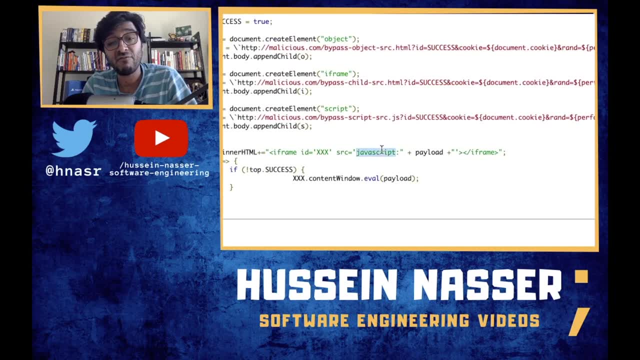 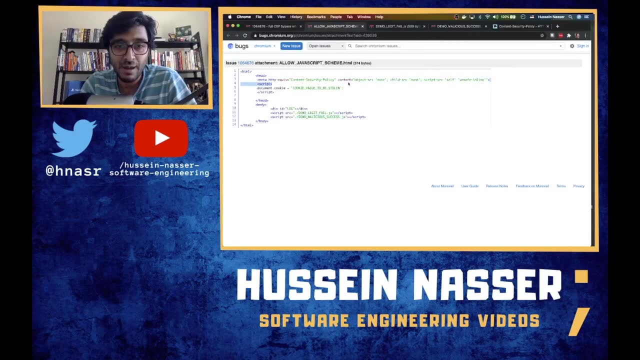 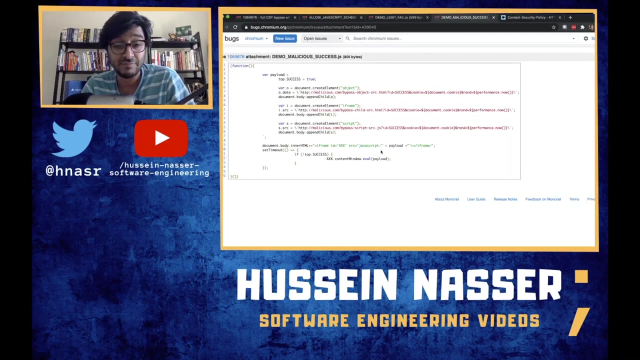 you can actually execute JavaScript code right there, But this actually becomes in a different page. They used that flaw because it's a new page. it's a new document. It did not inherit this content security policy, So pretty much it's a blank new slate As a result. 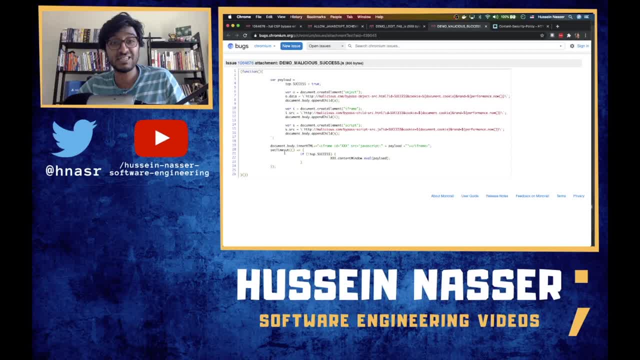 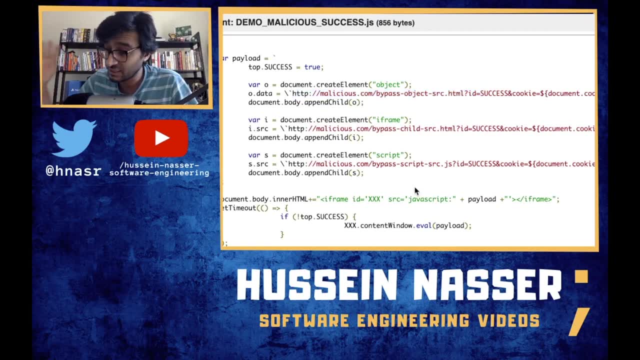 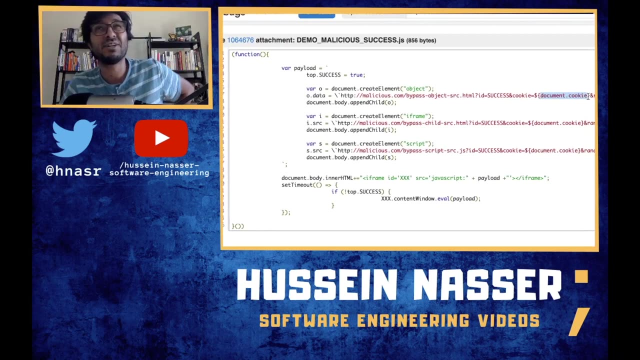 it's a blank slate and it will basically execute all that stuff. Execute this code and it will basically go to the malicious side. It will send the cookies. Now the question is: how did it have access to the cookie is beyond me, because it's a brand. 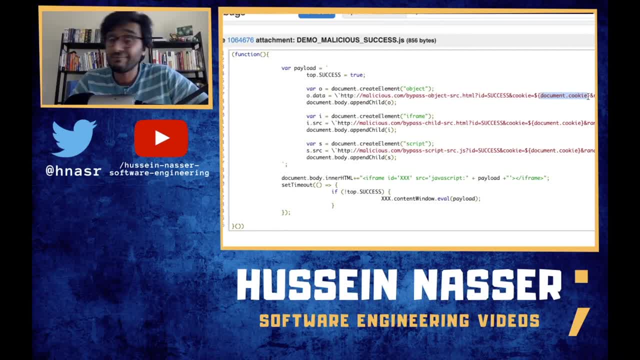 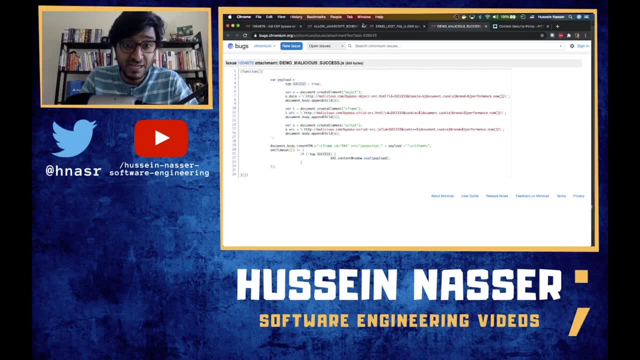 new page. I guess the brand new page will have access to that cookie. So yeah, maybe. So yeah, that's in a nutshell. that's the bug. It was fixed. That's why I was able to talk about it now. But look at this, guys. 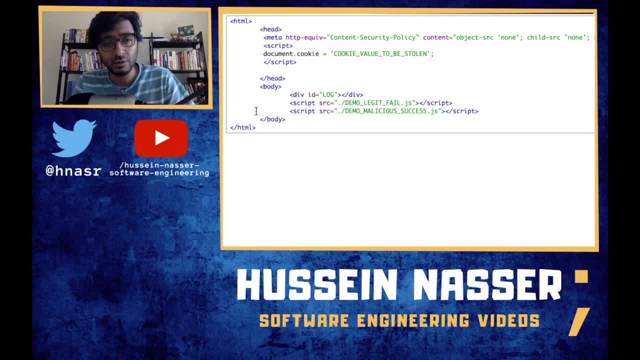 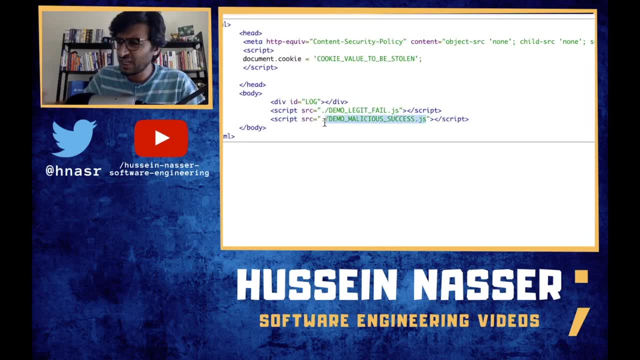 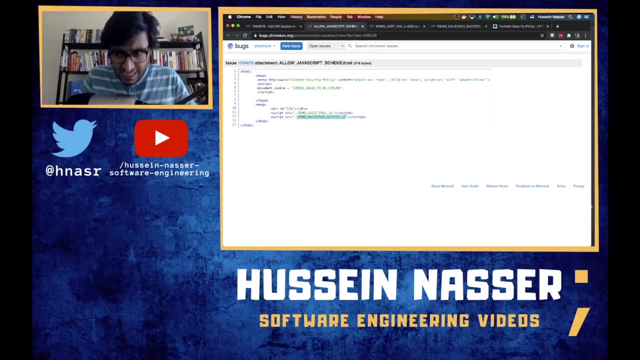 First of all, what did they have to do in order to execute this stuff? Well, they had to create a script and somehow inject it into my site. right, Because this script, that bad script, you cannot inject it in the page as a just normal script script. right, Because? 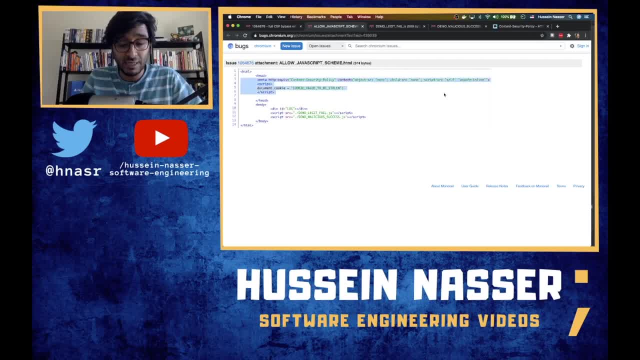 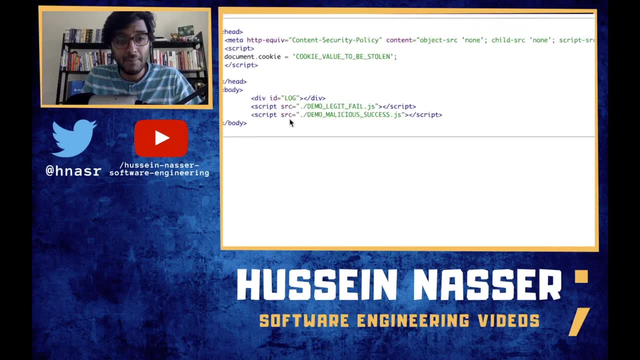 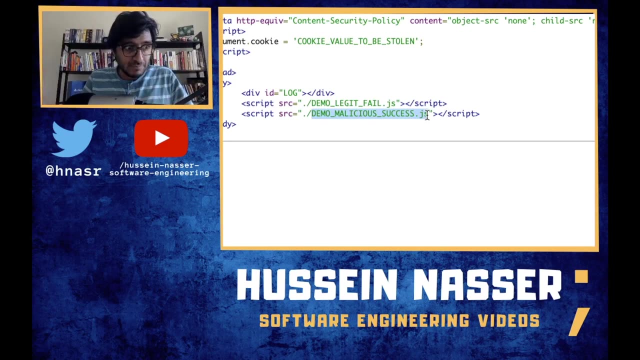 it will fail, right, Because we said unsafe inline. You cannot do inline scripts, right, So they cannot do that, So they should have been able somehow to make this work. You need to upload a JavaScript file to that web server hosting this content, And not only that, and modify, then do an XSS attack. 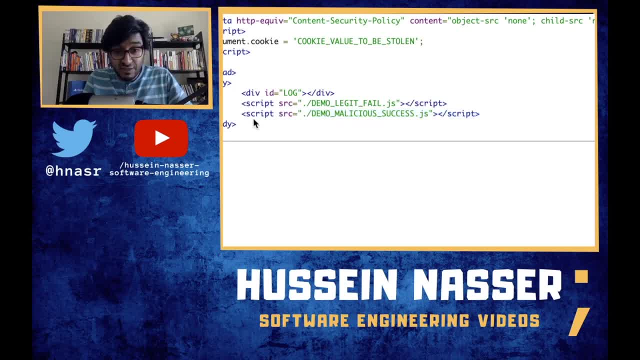 to inject a script tag that references that file you just uploaded. And you might say: how the heck can you allow people to upload a JavaScript file? Well, you can have a flaw in your uploading. You allow upload images, for example, and someone could just upload a normal ping or 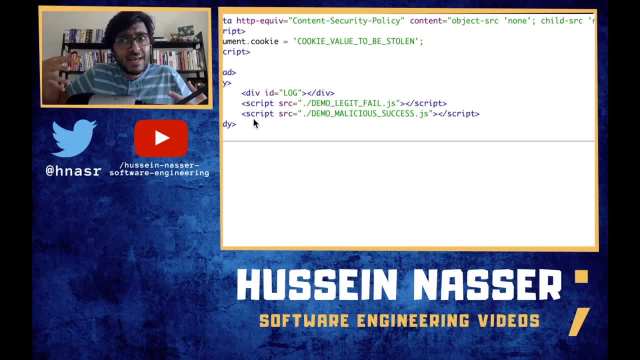 Jeff or GIF And that GIF or Jeff or image is actually a JavaScript file. But if your back end does not specify the content type of that ping file, because we don't know how to do that, we don't care about extensions- right The back end- Then if the browser tries to sniff, 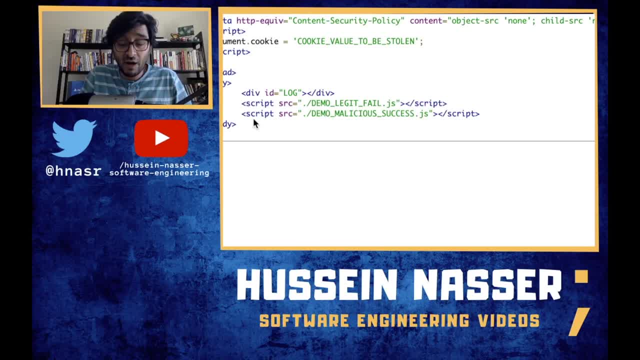 the content of the ping file, it can infer that the content is actually JavaScript and will treat it as JavaScript and it will essentially execute it right. So that's another way you can actually reference a job, an image here, and it will work as a JavaScript file. 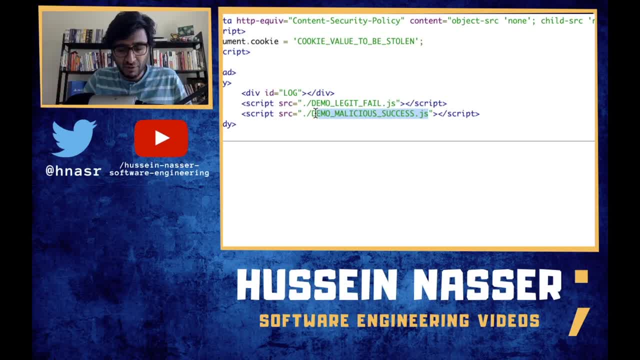 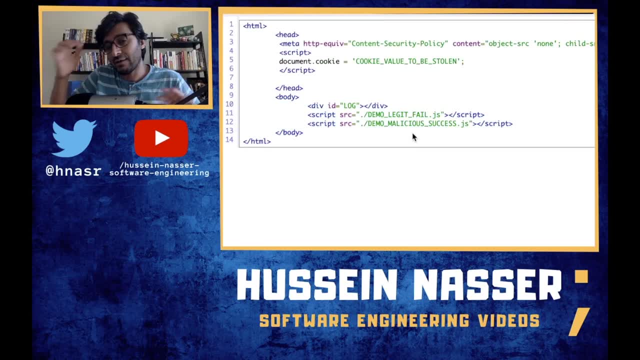 That's why you have to. I talked about- this is called mime sniffing right And I talked about my sniffing right here. Go check that video out. So that's another trick. If you're really a white hacker, white hat hacker, white hat hacker, is that right? Yeah, White hacker, You can actually. 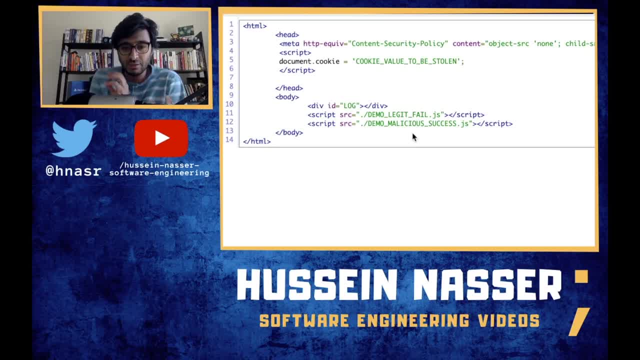 do all of that stuff and utilize all that stuff to fix your bug. That's why it's a complex field. You can just go into this back end security web stuff and and and you can still don't know everything. every day, man I I'm just amazed by how much I don't.